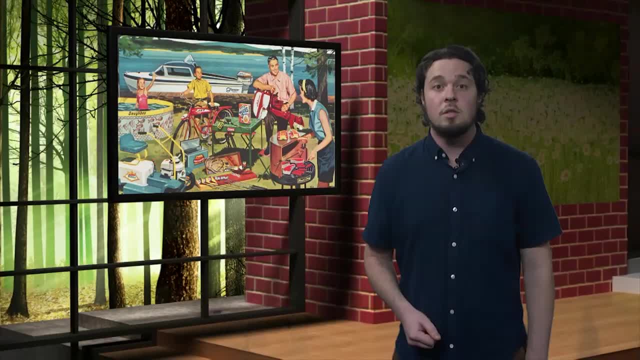 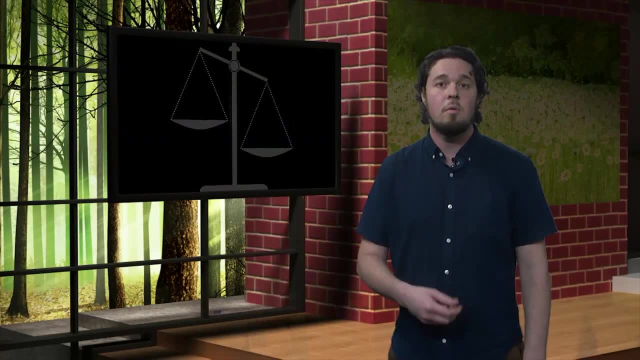 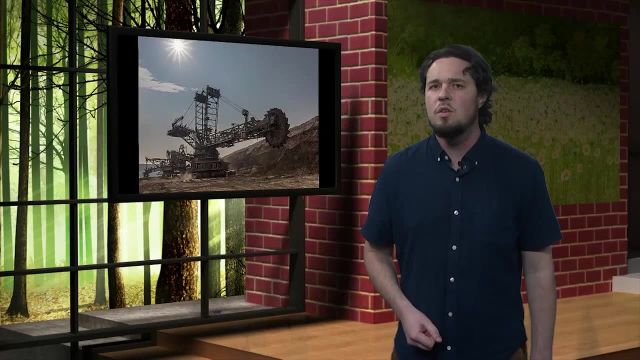 of environmental problems. Unlike shallow ecology, deep ecology emphasizes the cultural and ideological dimensions of ecological problems. For example, our socio-economic system may cultivate an attitude in which we view nature as merely an object that we can use For deep ecology. this attitude about our relationship toward nature is a 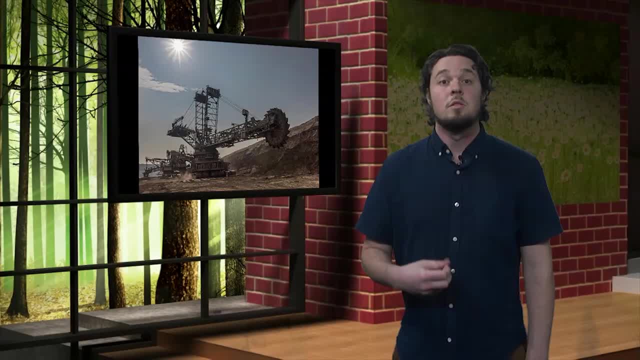 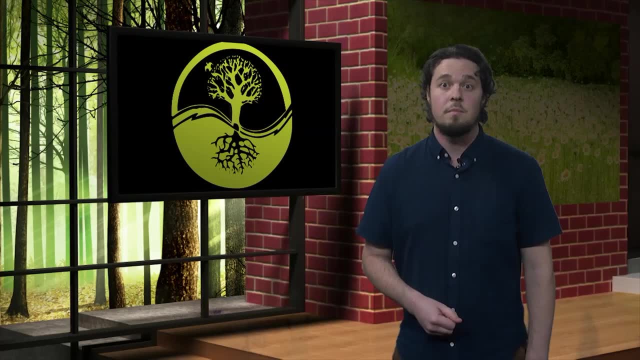 deeply rooted cause of environmental problems. So ultimately, people need to change their consciousness to address the root cause of environmental problems. Let's look at some examples. Let's look at this idea in more detail, For deep ecology, a common but mistaken view of our own nature is the fundamental cause of ecological problems. 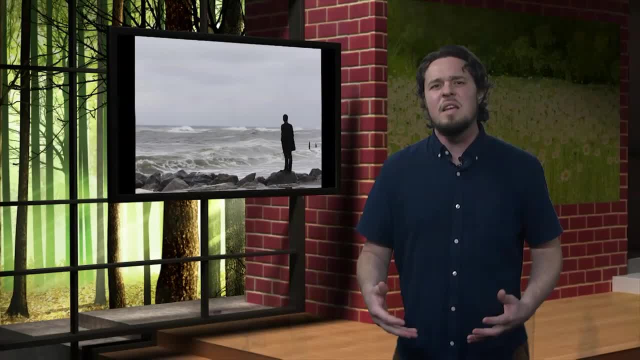 It's a mistake to view ourselves as distinct from the natural environment, and it's a mistake to conceive of our egos as atomistic and isolated from other beings. So, for the deep ecologist, addressing environmental problems ultimately requires correcting this view by attaining a deeper understanding of the nature. 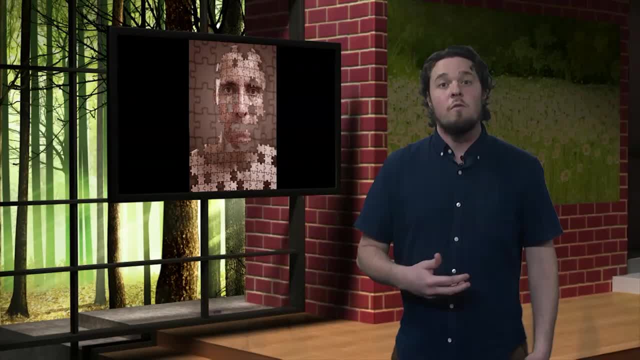 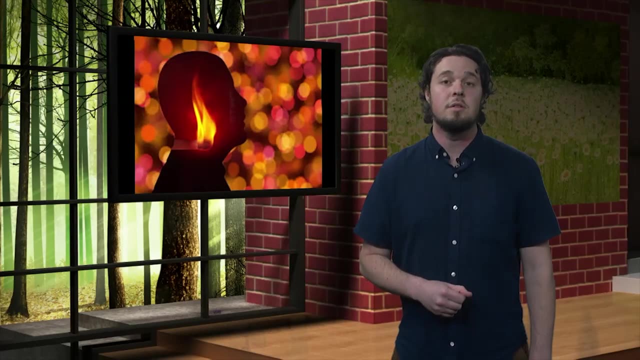 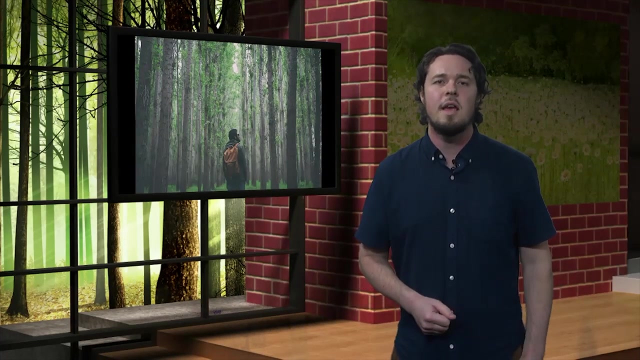 Now, unfortunately, correcting this misunderstanding of our nature will be difficult, since it's deeply ingrained in our culture. According to deep ecology, pursuing self-realization is the key to understanding our true nature. In this process, we gradually become aware of ourselves as fundamentally interconnected with everything in nature. 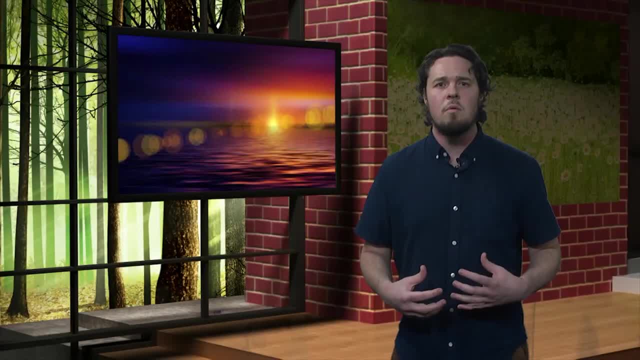 We start to see ourselves as more than a narrow ego and we begin to identify ourselves as a narrow ego. We begin to identify ourselves as a narrow ego and we begin to identify ourselves as a narrow ego. We begin to identify ourselves as a narrow ego and we begin to identify ourselves as a narrow ego. 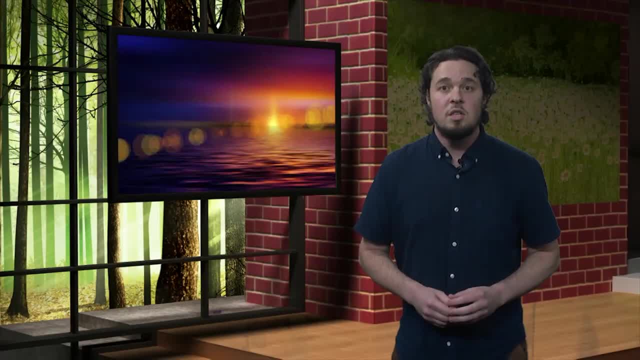 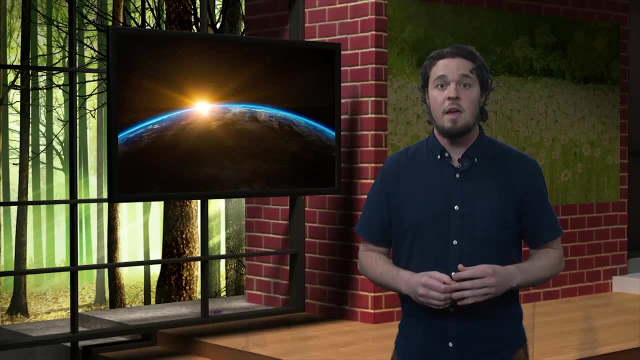 We begin to identify ourselves as a narrow ego. By self-realizing, we identify with all other beings. We begin to see ourselves as an ecological self. As Arnie Iness puts it, the ecological self is a self that is in of and for nature. 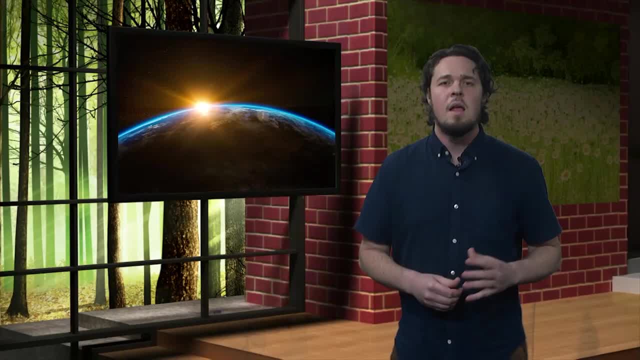 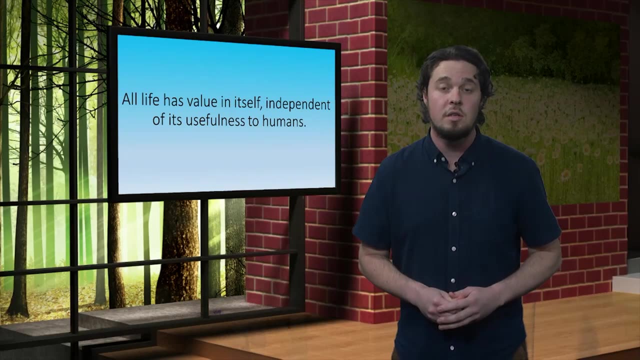 Now for philosophers Arnie Iness and George Sessions. this ecological understanding of ourselves supports eight principles of deep ecology. First, all life has value in itself, independent of its usefulness to humans. to humans, Second, richness and diversity of life helps the realization of these.